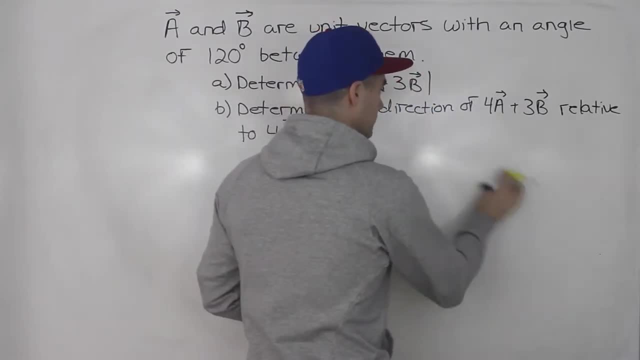 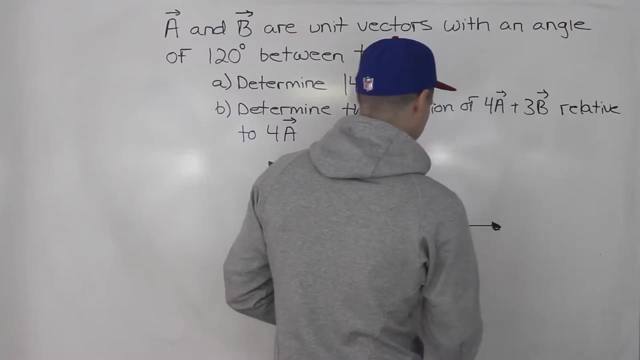 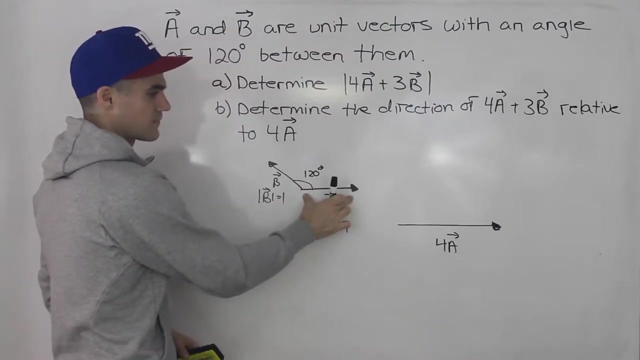 let's say, actually, let's draw it a little lower. So let's say this: right, here is 4a, Right? so I just took this vector and then extended it four times. Now it's not necessarily to scale, but let's just pretend this vector is four times the length of this one, four times the. 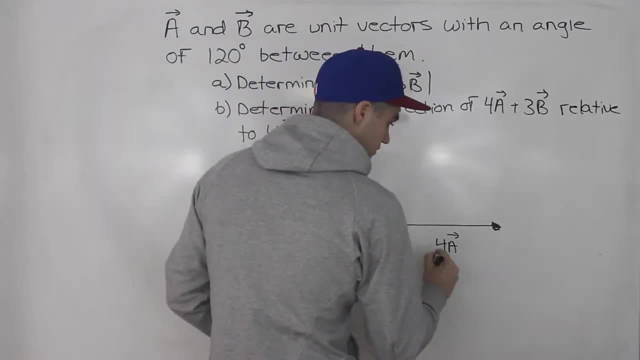 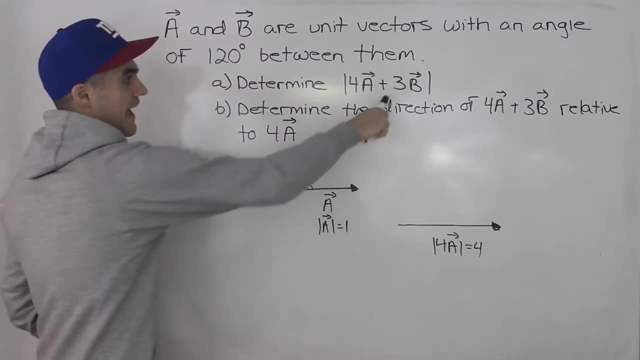 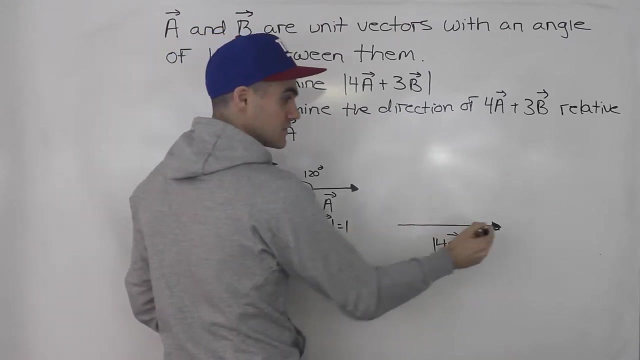 magnitude. Four times the magnitude means the magnitude of this vector is four times the magnitude of this vector. The magnitude of this is going to be four, And then we have to add 3b to it. Now, when we're adding vectors, we have to add the tail of the next vector to the head of the previous vector. 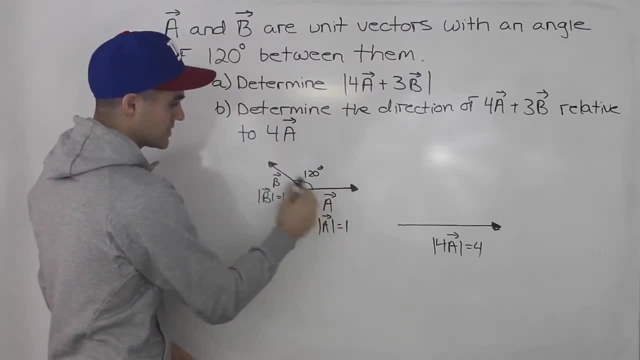 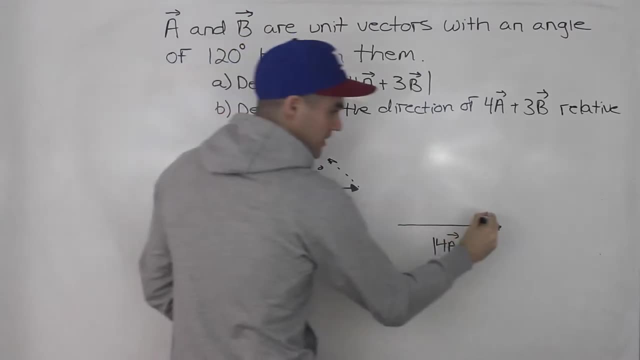 So notice, this is tail to tail. so if we were adding these two like a plus b, we would have to take this vector and shift it like that. So when we're adding 3b, instead of it being tail to tail, we would shift it and it would go this way: 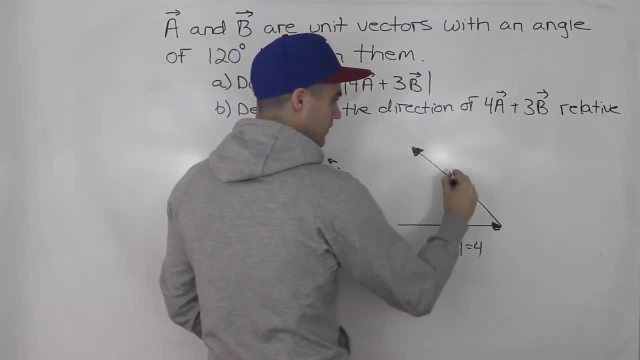 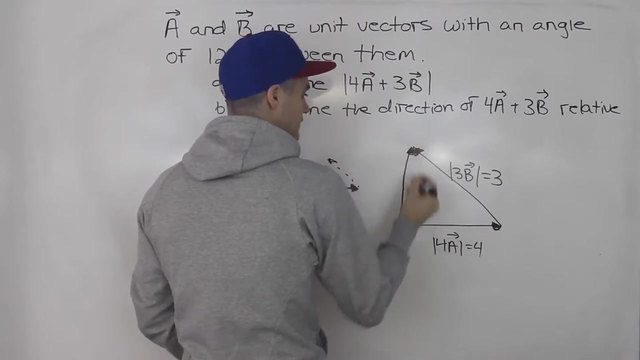 like this. Right, so this would represent 3b over here, and because vector B is the unit vector, the magnitude of this is going to be 3.. Right, so this vector, the resultant from the tail of the first vector to the head of the last vector, this vector here, 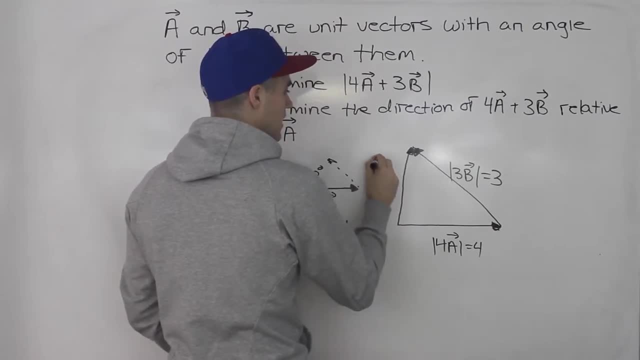 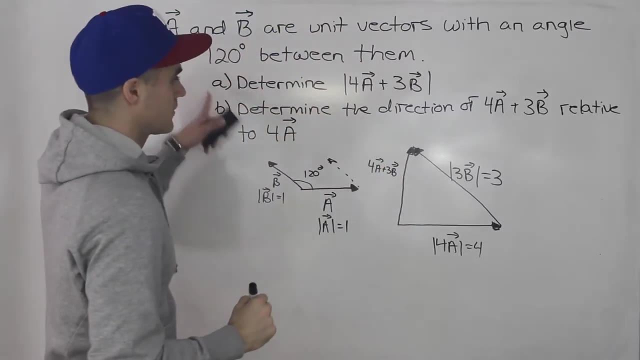 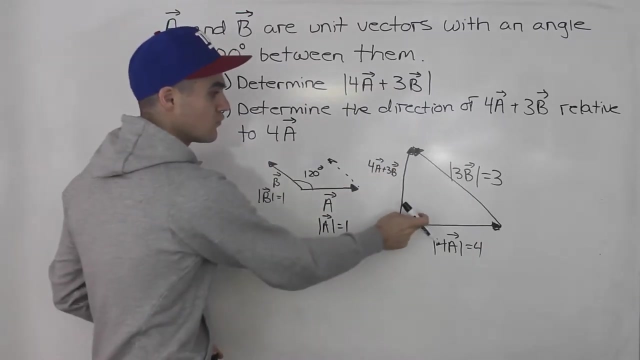 right From the tail of the first vector to the head of the last vector. this vector here represents 4a plus 3b, this vector right here. so in part a we have to determine what is the magnitude of this and then for part b we have to determine the direction of this vector: 4a plus 3b relative to 4a. so we're. 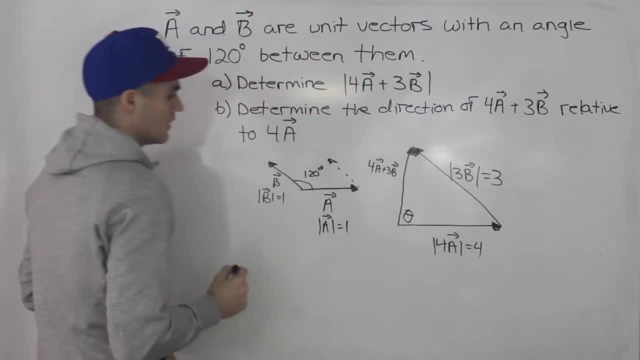 going to have to solve for this angle over here, right? so going back to this, notice that the angle between these two vectors is 120 degrees when they're tail to tail. so if we take this vector and we sort of shift it over, that means that this angle is going to be the same as that. 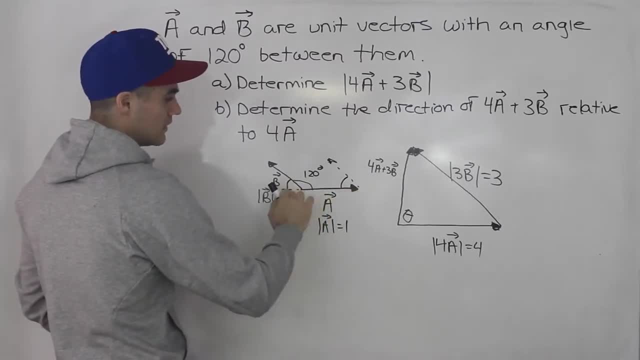 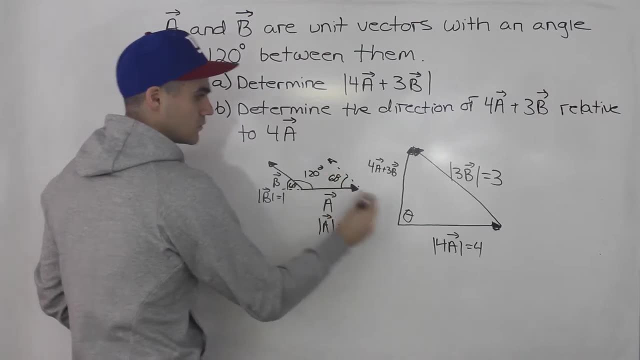 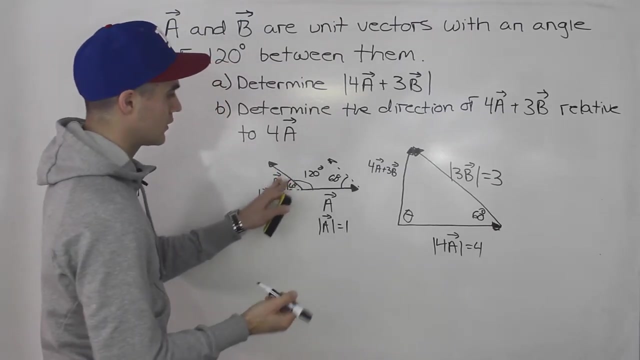 angle right, because it's just a parallel line here that's extended. so if this whole thing is 180 degrees, this is 120. that means this is going to be 60, which means that this here is going to be 60, right. so there was an angle of 120 degrees between them, but 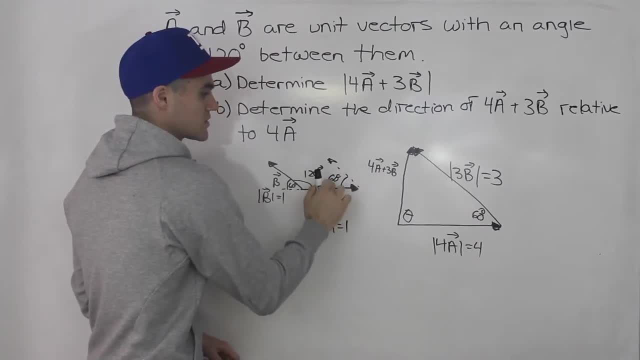 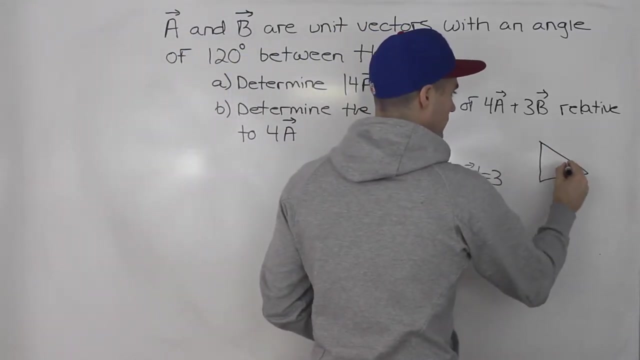 when we shift it with that z pattern, 180 minus 120 gives us 60. so now notice that we just have a triangle. right, we have a triangle where, if i draw a smaller one out, we have an angle 60 degrees. here we got three, we got four. 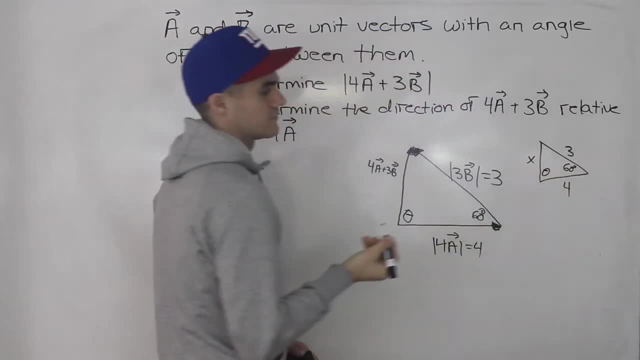 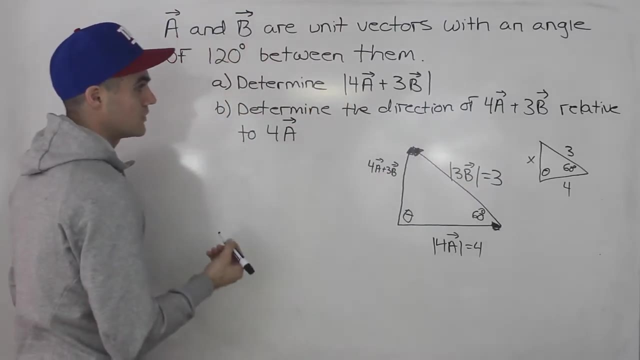 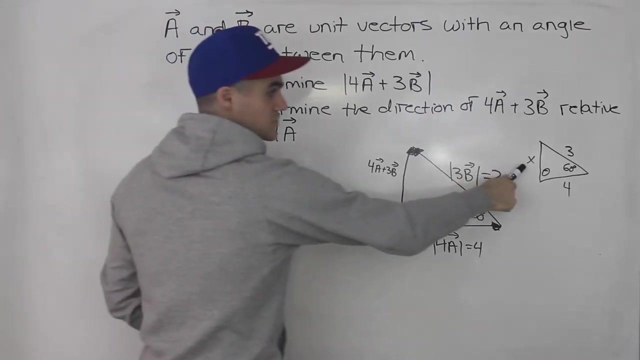 and we're solving for x and theta. that's pretty much it. so to solve for this x, which is the magnitude of this vector, 4a plus 3b, what would we do? we would use cosine laws. so for part a we'll have x squared right. so i'm just using the notation from this triangle. it's equal to: 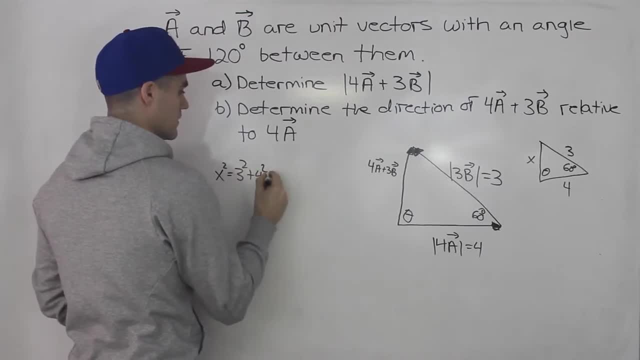 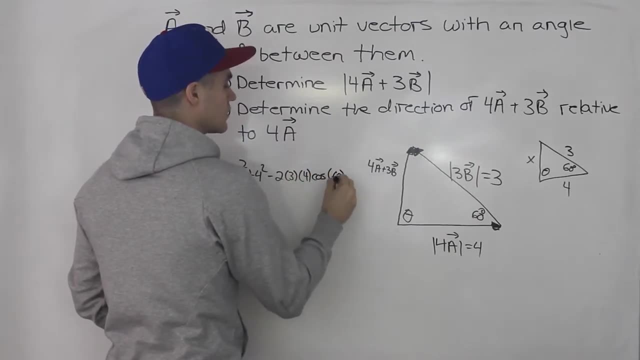 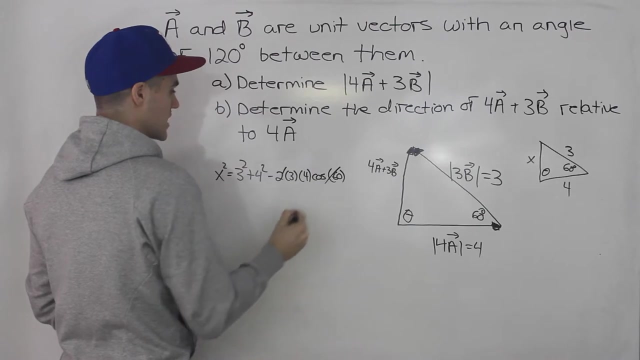 three squared plus four squared minus two times three times four times, cos, uh, of 60? close of that opposite angle, and we know cos of 60 is one half. so one half times two, those will just cancel out. so we'll have 9 plus 16 minus 12, that's equal to x squared. so that means 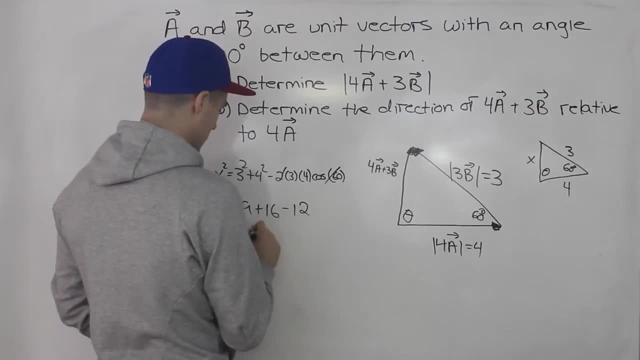 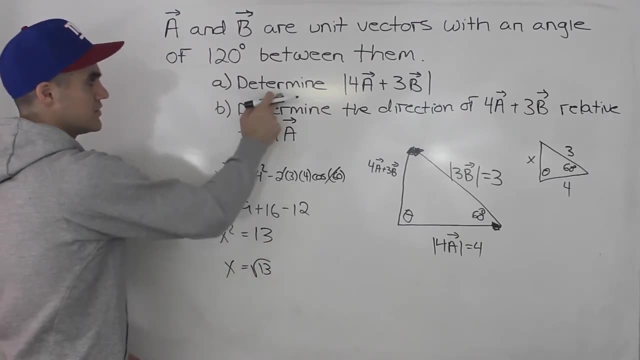 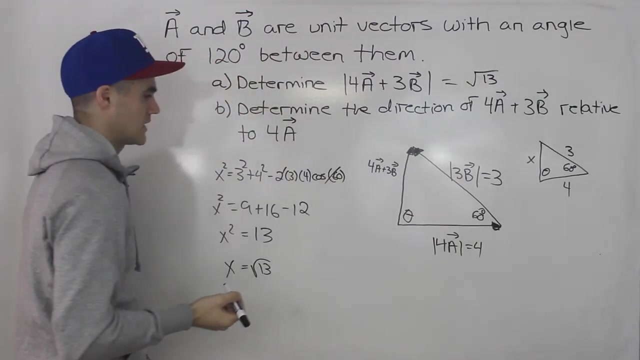 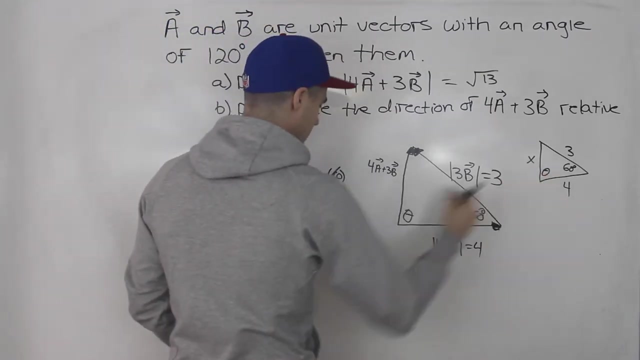 x squared, 9 plus 16 is 25 minus 12 is 13. so x is root 13. so the answer to part a, the magnitude of this vector, is root 13, like that. and now notice that we can solve for this theta as well. we can just use sign law now, so we would have sine of 60. 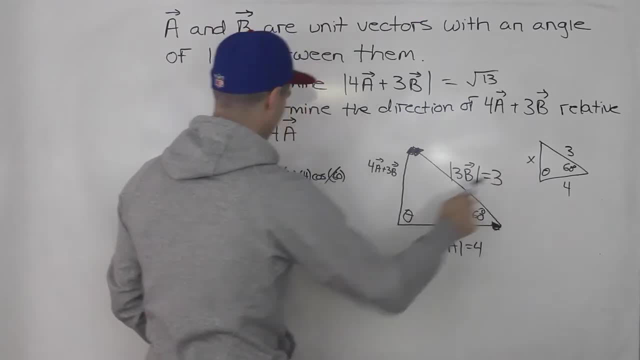 over x. x, we know, is root 13 equals sine of theta over 3, and now we just got to solve for that sine of theta. so we're going to solve for those 여기까지 with an international number of anyway. and then the magnitude of this vector is: Tenemos que la velocidad, is read threat like that. and now notice that we can solve for this theta as well. we can just use sign law now. so we would have sine of 60 over x, approximately, or 30 over x squared, equals sine of theta over 30. 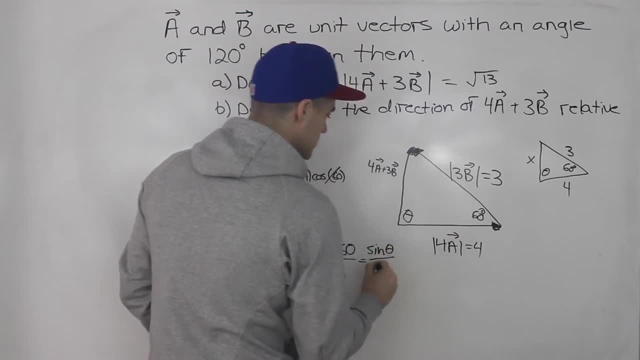 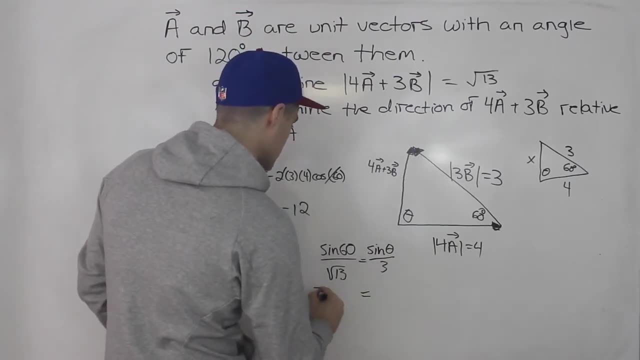 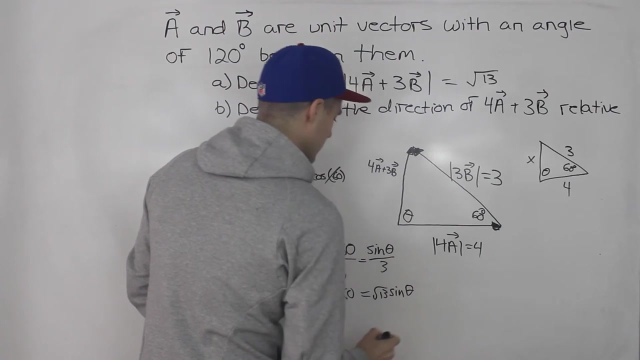 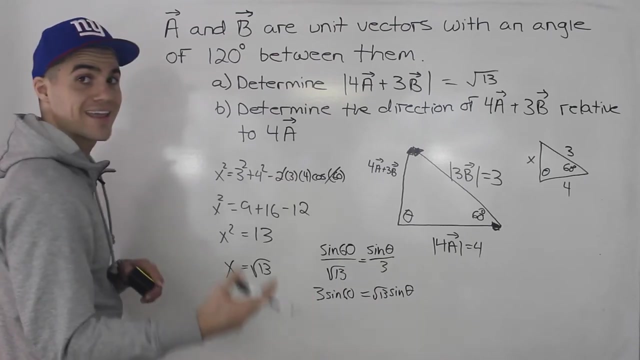 and now we just got to solve for that sine of theta. so when we cross multiply we would end up having what's 3 sine 60 times root 13 sine theta, and then we would divide both sides by root 13 to get that sine theta by itself, and then inverse.